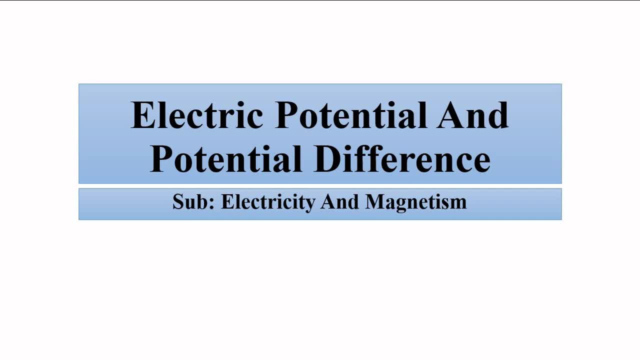 uniformly charged circular ring and various other introductory concepts related to that. So in this video we are going to discuss about electric potential and the concept of potential difference. ok, So everything related to you know electricity. it has one common thing which is associated with it. 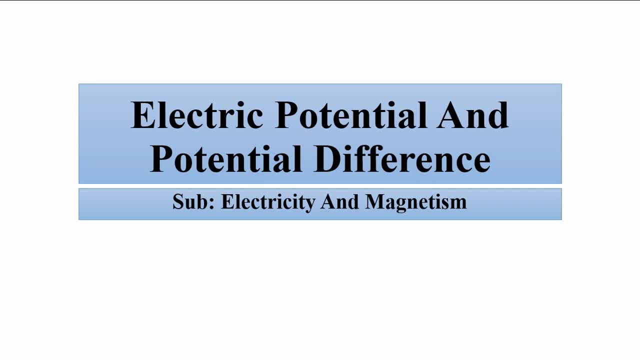 Which is the, the source of that which is charge. ok, Charge from charge. first we discussed about the fundamental concept related to charge from charge. we went to, you know, Coulomb's law. from Coulomb's law, we went to electric field, and then from electric field we carry out our discussion. 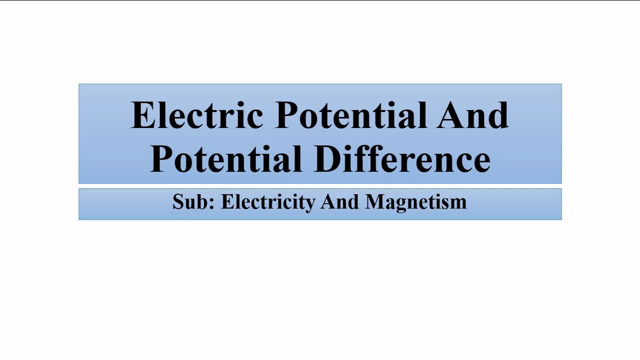 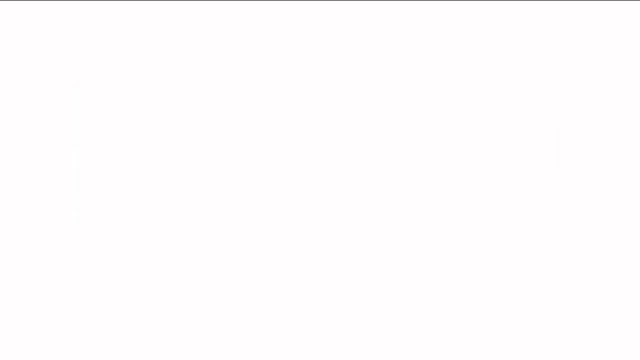 forward. So before discussing electric potential and potential difference, first we have to discuss about one important thing, which is the potential energy of a charged particle in an electric field, or we can write it as electrostatic potential energy. This, ok, So the potential energy of a charged particle in an electric field, we can correlate. 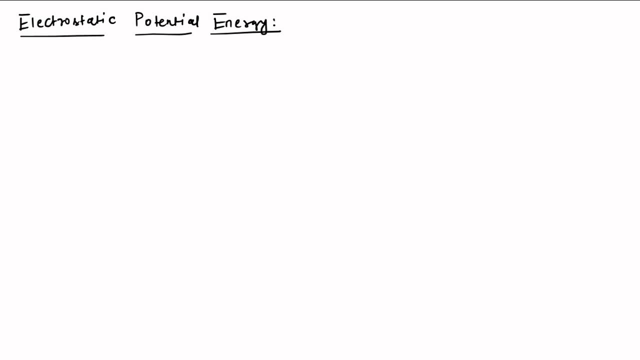 with it with the potential energy of a mass. ok, in the gravitational field, Suppose we have A mass m, ok, and it is located at a distance or a height of h from the ground. ok, So here the potential energy of this mass is given by the formula m, g, h. Mass acceleration ratio. 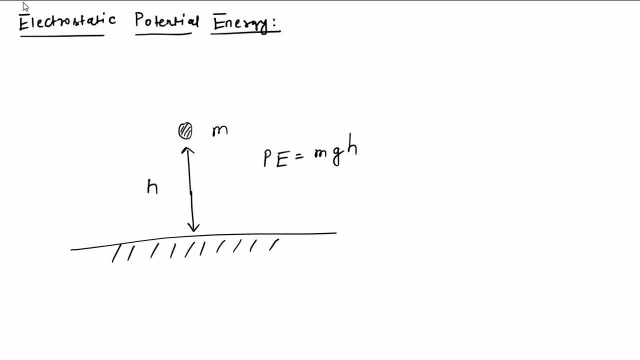 due to gravity, which is 9.8 meter per second square, and then we have the height that similarly, this is the gravitational potential energy, or simply it is also called as gravitational energy in the electrostatic field. the same discussion, if we convert it or we take it to the electric field, in that 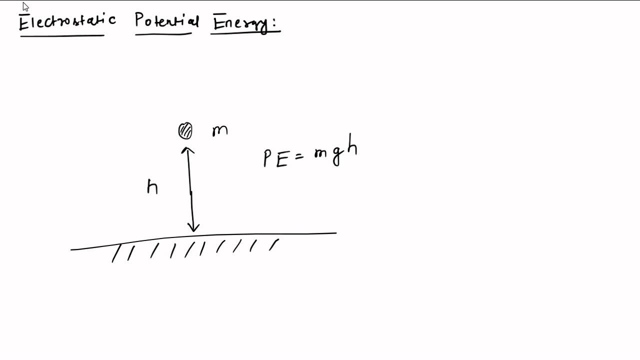 case, the mass can be replaced with charge, the gravitational field can be replaced with the electrostatic field. this, okay, and the potential energy which is there, it is called as the electrostatic potential energy. okay, so a charge in an electric field has electrostatic potential energy. in the same way, a mass has gravitational potential energy in a 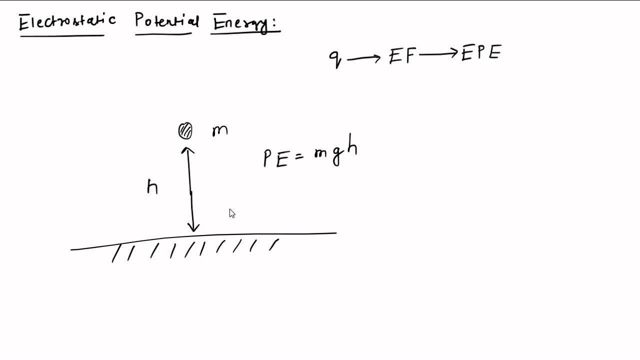 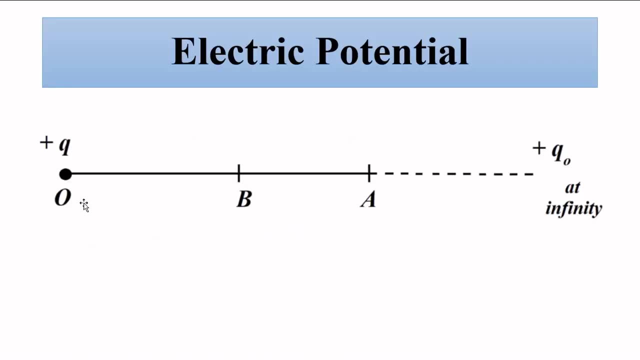 gravitational field. okay, so in order to understand this concept, first let us say the same thing, same thing. we have a point charge, let's say plus Q- positive charge- located at O, and then we have a test charge- Q zero- located very far away from it, theoretically at infinity. 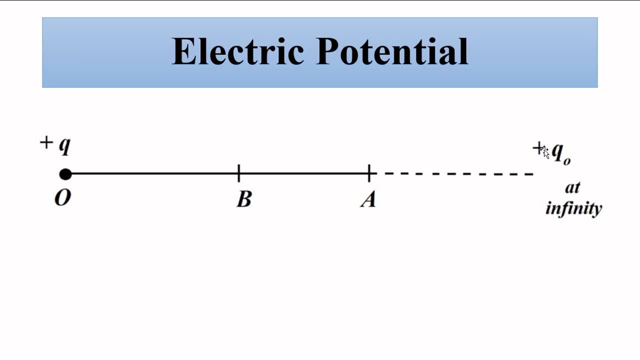 so, at infinity, the test charge which is located, it has, or it is assumed to have, zero electrostatic potential energy. okay, at infinity, this test charge has 0 electrostatic potential energy. it is 0 at infinity. this Now, as this test charge is moved from this far away distance from infinity towards this: 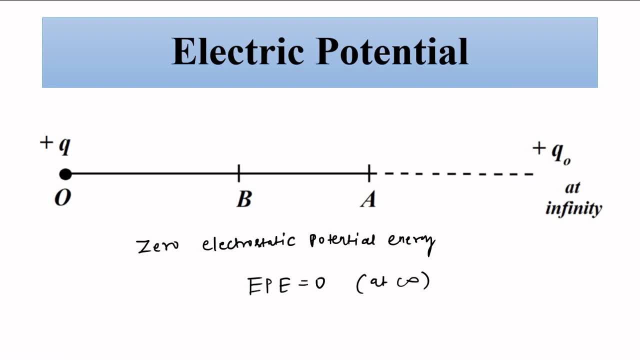 plus Q charge at a uniform velocity. there will be some work which has to be done Now. both these charges- the original charge, the source charge and the test charge- they are positive, So it will exert a Coulombic force of repulsion on this test charge. 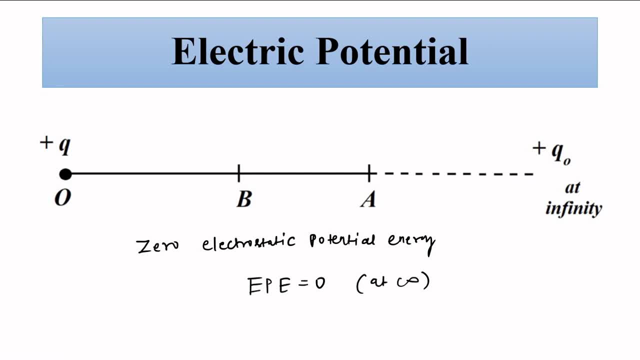 So it has to be moved against the electric force of repulsion to move it closer to the closer to O. So that work which is done to move this test charge closer to point O, closer to the source charge that is stored in this charge as electrostatic potential. 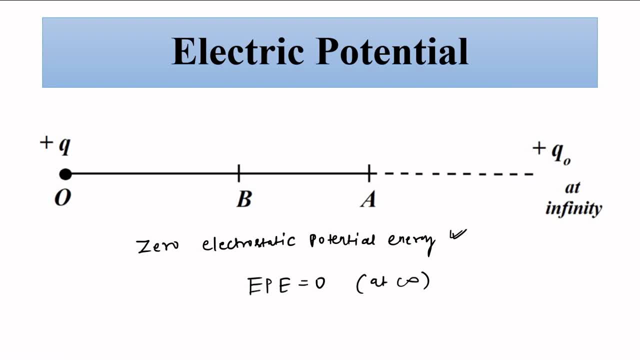 energy that. So electrostatic potential energy is the work done against the electric force of repulsion to move the test charge closer to the source. Okay, source charge that. So here let us say that we have this test charge at infinity, and let 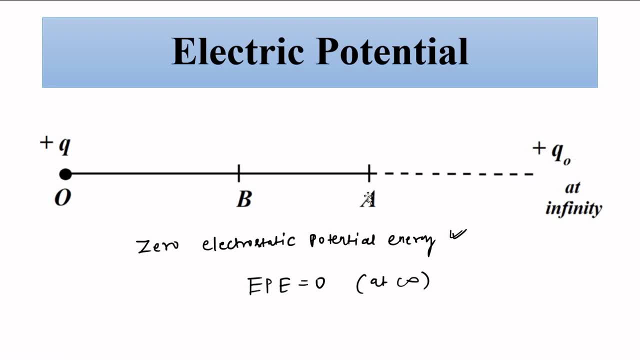 us say it is moved to this position A. So the potential energy of this test charge at A, let us say we call it u A, It is the work done in moving the test charge from infinity to A. Similarly, the potential energy of this test charge plus q, 0 at B is the work done. 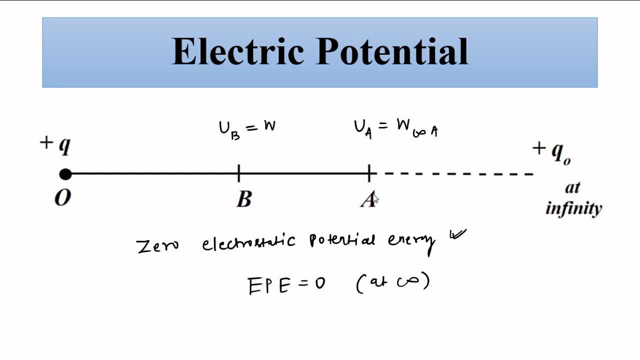 in moving the charge from infinity to B. Now, as B is more closed, Closer to the source charge or more closer to the point O, So more work will be done to move the charge to the point B, then the to move it to point A. So obviously u B. 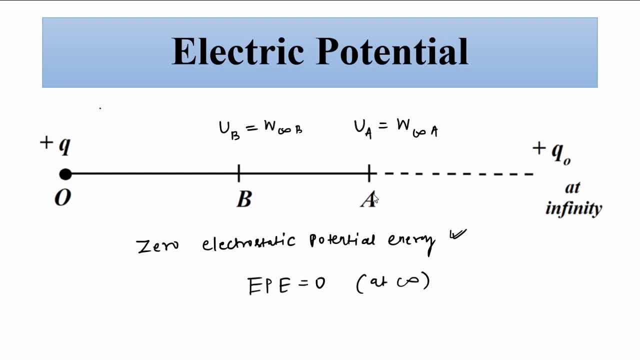 will be greater than u. A potential energy at B will be more than potential energy at A, because more work will be done to move this test charge to B, which is closer to O, than the work Which has To be done to move it to A. So the work done in moving the charge from infinity to B is 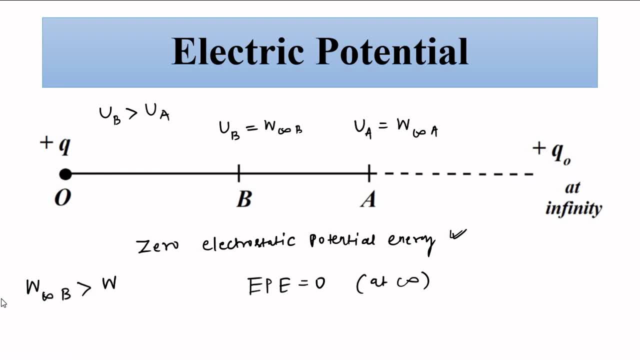 greater than the work done in moving the test charge from infinity to A. So this is the concept of electrostatic potential: energy. This now comes the turn of electric potential. So, for electric potential, what we have to do is that, like the electric field, in electric field, in order to define electric field, we 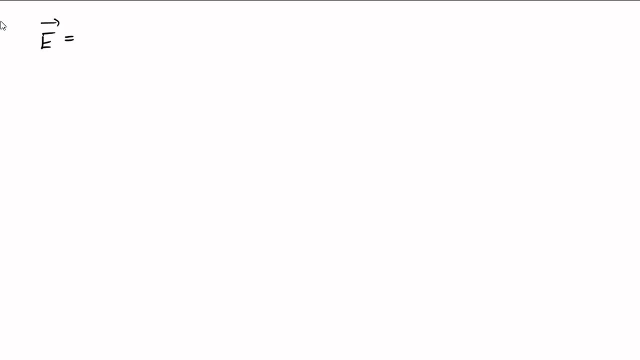 had the force which was exerted on the test charge q 0, it was divided by the test charge itself, The coulombic force divided by the test charge. here, in order to find out the electric potential, what we have to do Is that: 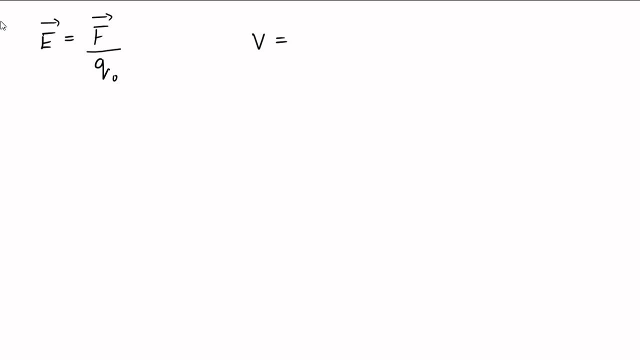 Is that we have to divide the work done, or work which was done to move that test charge closer to the source charge, divided by the test charge itself. there it was. in electric field it is forced by test charge. here it is work done on the test charge in moving. 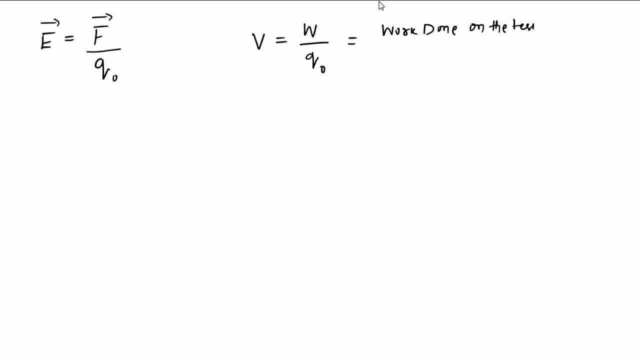 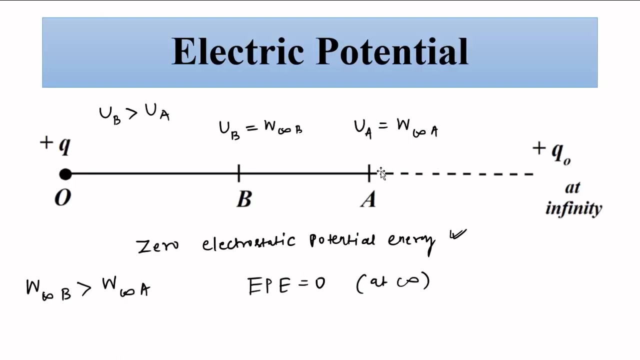 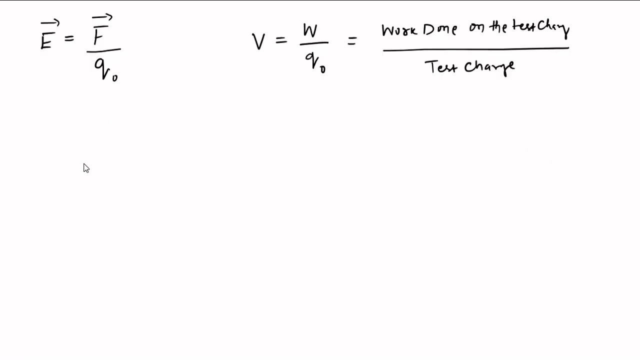 the test charge. So that is the point A divided by the magnitude of the test charge at the ok. this So here, in this case, the electric potential at the point A- ok, the electric potential at point A is simply the work done. electric potential at point A, let us call it V, subscript A, The 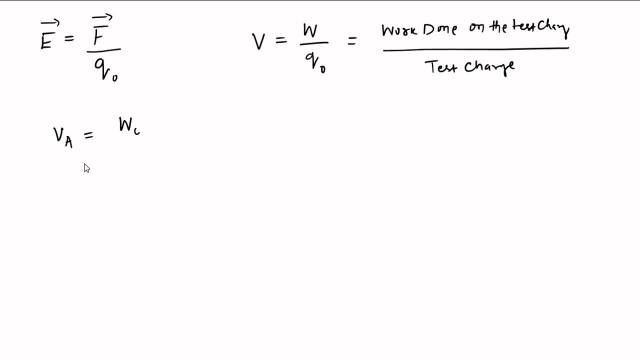 work done, moving the charge from infinity to point A divided by the test charge value, or which is simply the electrostatic potential energy of the test charge at point A divided by q0, and similarly, the electric potential of the test charge at this point B: electric potential. 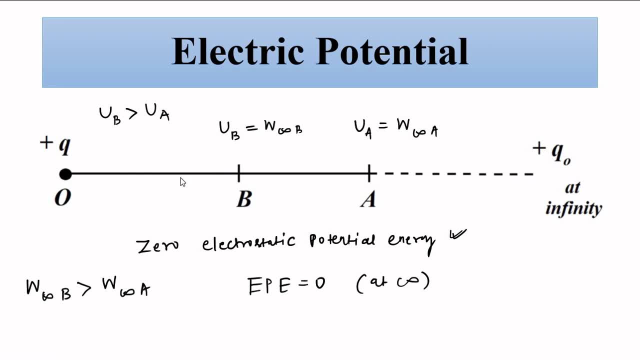 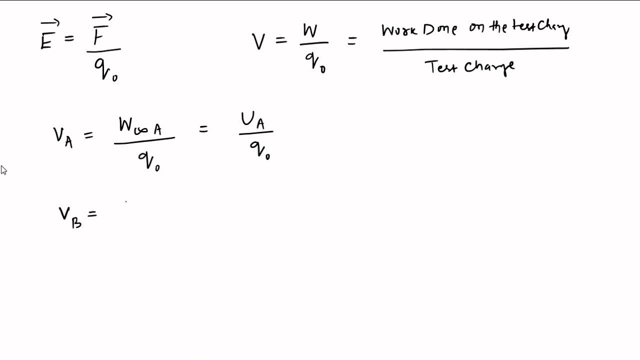 at B is given by VB, The work done in moving the test charge q0 from infinity to B divided by the test charge value, which is the electrostatic potential energy of the test charge q0 at point B divided by q0.. So here in order to define, be it electric field or be it electric, 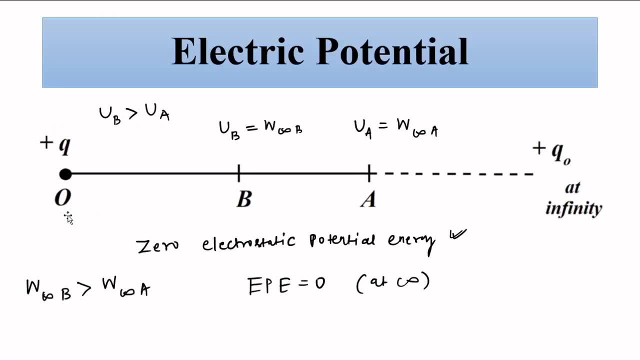 potential. There are two things Which are always important. first, the source of the electric field or whatever which is producing the source, that is, the source charge and the test charge. So it is always relative to these two things that everything associated with electricity it is defined, be it anything. 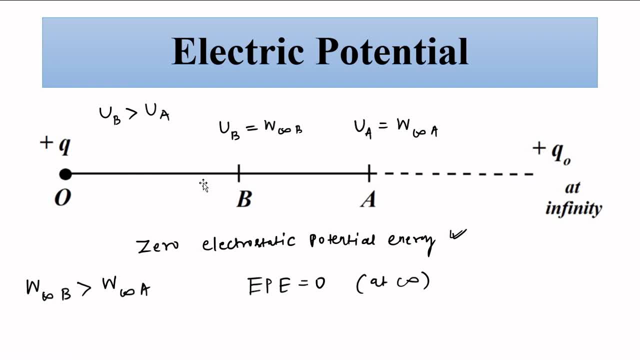 coulomb, coulomb slow, the coulombic force, electric field, electric potential, everything. So electric potential is simply the work which has to be done on the test charge to move it closer to the source charge against the force of coulombic force of repulsion divided by the 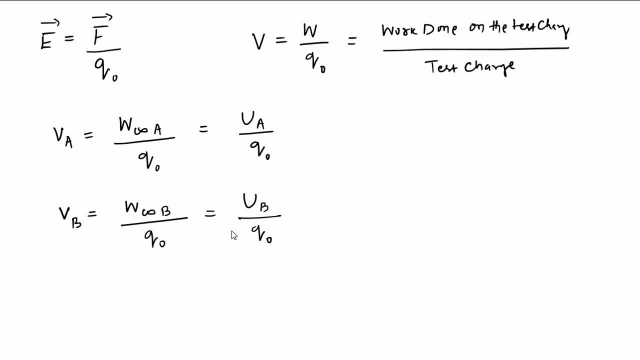 value of the test charge itself. So if we consider a unit positive test charge, that is, the value of q 0 is 1 coulomb, Then will have V A as W F phi A or U A, and V B is equal to W phi B or U B. this ok, So the 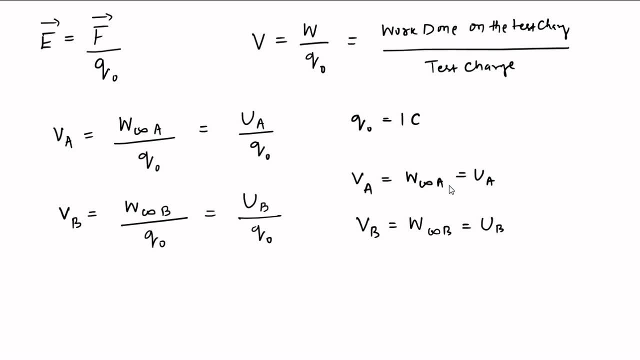 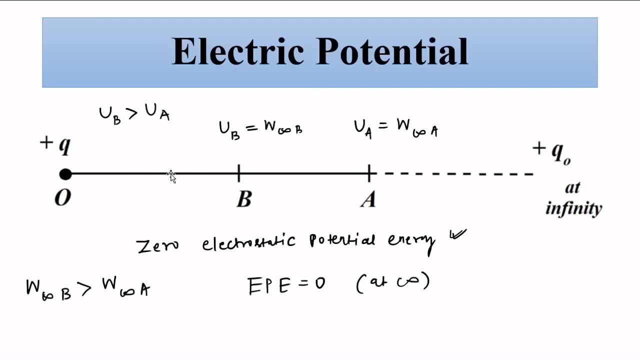 electric potential at any point in an electric field- ok, at any point in an electric field- is simply the amount of work which has to be done in moving a unique positive test charge from infinity or a far away distance to that point, to that particular point, against the 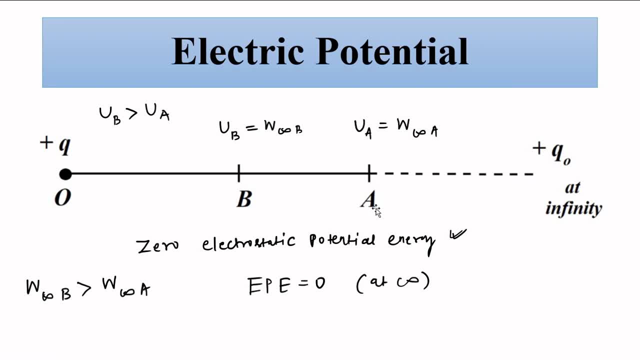 electrostatic force of repulsion. ok, Here both are positive, so there is a force of repulsion. if it would have been opposite charge, then it would have been attractive force. ok, So electric potential is simply work done by charge. ok, So here we can also write as the potential energy. 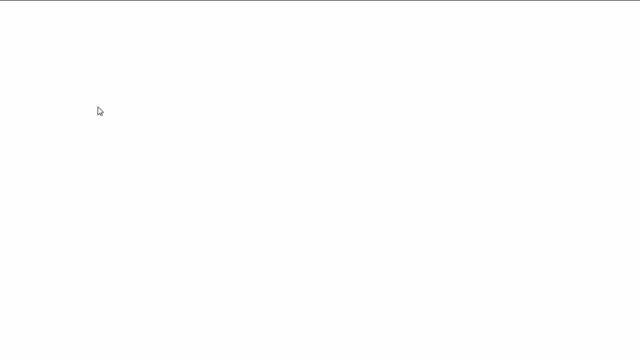 U ok potential energy we are. the electric potential which is defined at any point, is simply the work done By charge, or the electrostatic potential energy divided by the charge U by Q. So we can write the electrostatic potential energy as Q- V, product of the charge and the electric potential. 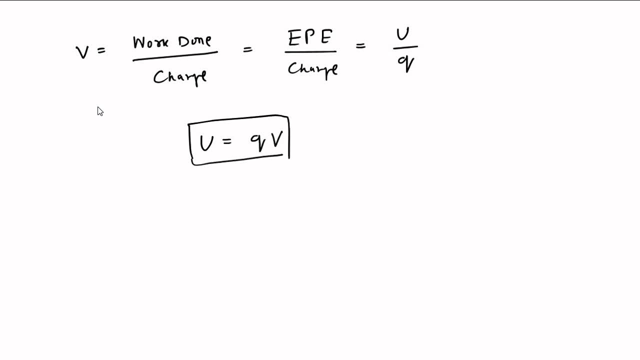 ok, The SI unit of electric potential. it is defined in terms of volts, the unit of electric potential. for electric potential, the unit which is defined is volt, ok, volt. So this means that the unit or the SI unit of electric potential, 1 volt means 1 joule. 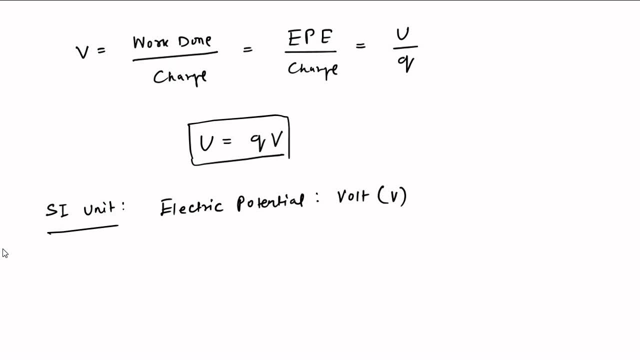 of work is done to move a charge of 1 coulomb against the electrostatic force. ok, 1 joule of work is done in bringing a unique positive charge, that is 1 coulomb plus 1 coulomb of charge from infinity to that particular point against the electrostatic force that 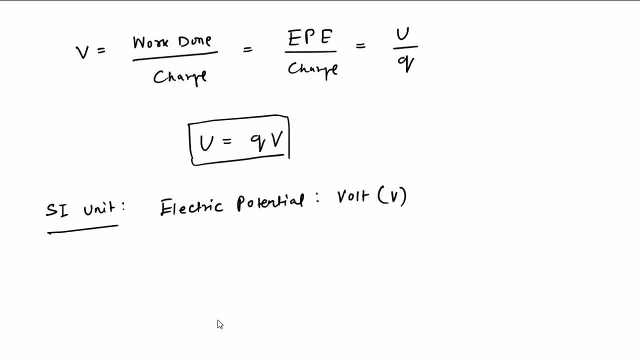 means 1 volt. So 1 volt simply means 1 joule of work is done for that. ok, 1 joule of work is done to move 1 coulomb of charge from infinity to any particular point on the electrical field. ok, 1 joule by 1 coulomb, that is 1 volt, ok. 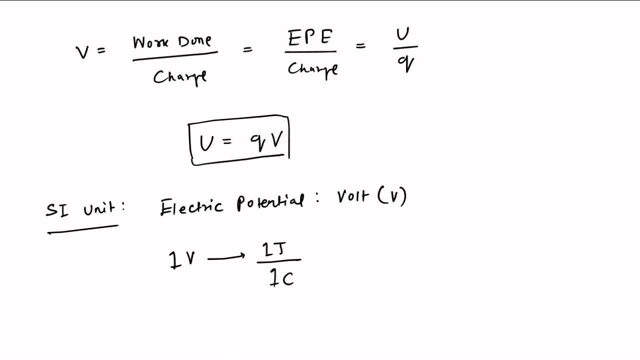 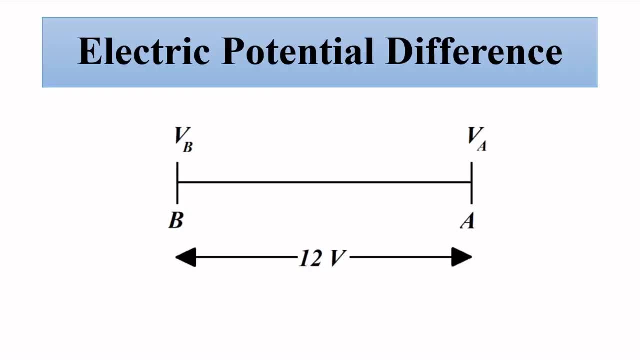 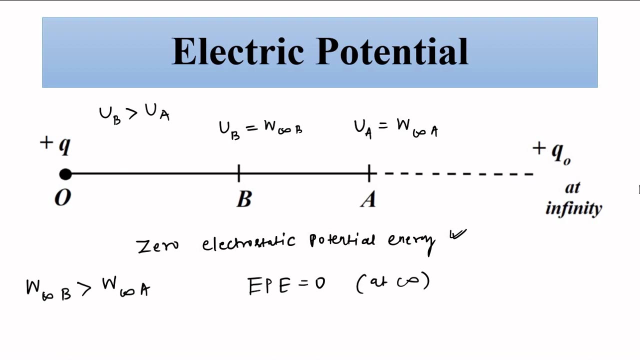 Now electrostatic potential difference, electric potential difference between any two points. So electric potential is defined at any particular point with respect to infinity. ok, from infinity to that point, that is electric potential. 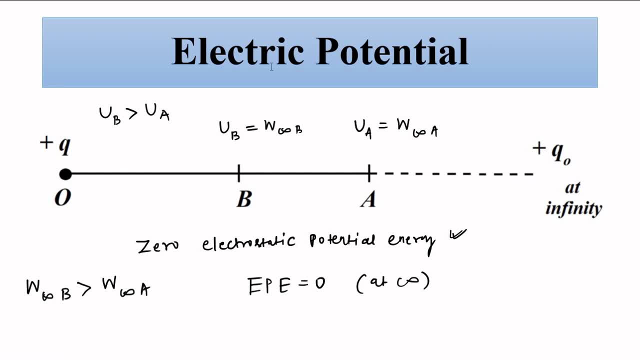 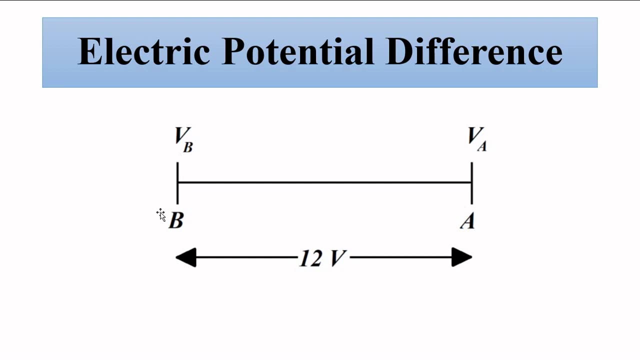 Perfect, That is 1 volt. So here let us say, for example, we say that the electric potential difference 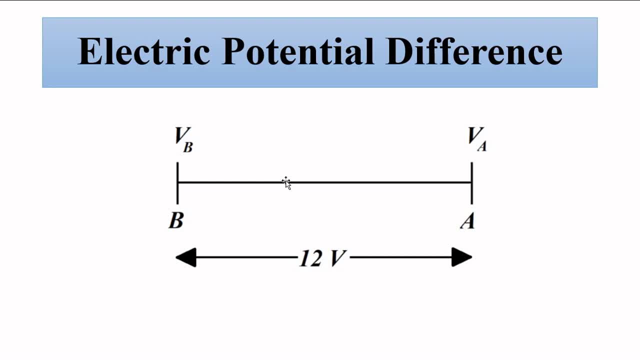 between points A and B is 12 volt. ok, it is 12 volt. it means that first we have to define this point. we have this point at infinity. we have a test charge here. So it means this test charge, which. 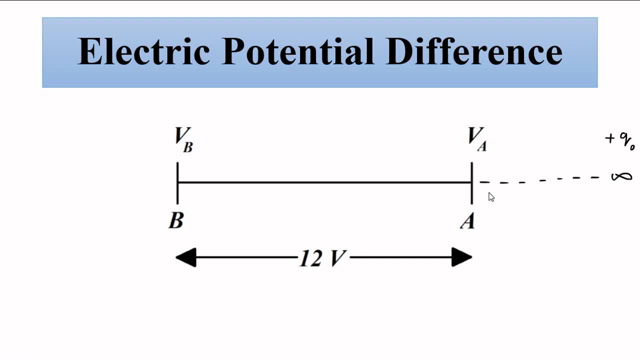 was originally located at q0, the work which had to be done to bring it from this infinite point to this point a. let us say that is w phi a, and then this test charge again. if, when it has to be moved from this point to this point, it is w phi b, It is. we can also write it as u a, this we can. 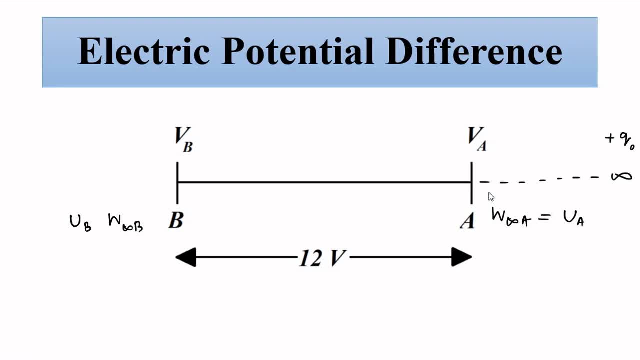 write as u b. Now v b is simply w phi b by q0 and v a is w phi a by q0. Now u b is greater than u a, So obviously v b will be greater than v a. So here potential. 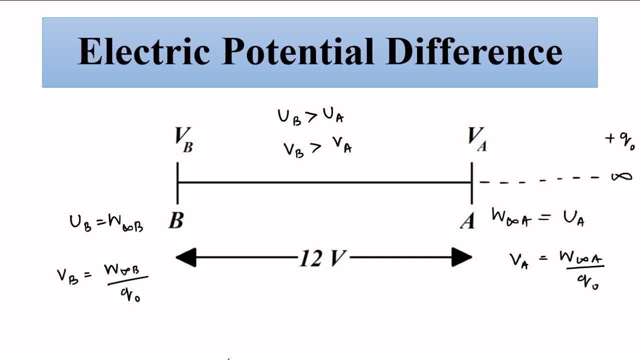 difference between these two points, b and a, is simply v b minus v a, which is w phi b by q0 minus w phi a by q0, which is w phi b minus w phi a by q0. or we can say it as the work done in moving the test charge from a to b against the electrostatic force. 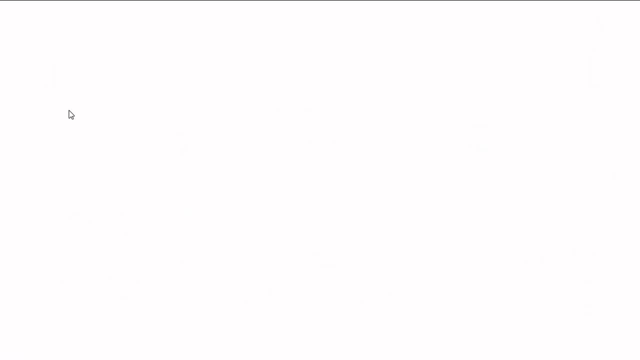 So the potential difference between these two points, or any two points, let us say the potential difference between point a, b and a, v, b minus v a, So the potential difference between these two points, a and b, b, being at higher potential. 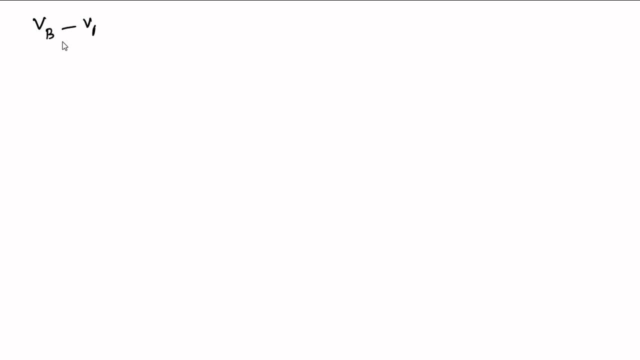 point at a. this is the work done in moving the charge. work done in moving the charge, the test charge, from a to b, That is, lower potential to higher potential. used to lower potential, point to higher potential. We can also write the next characteristic equation: So there is 1 by 2 if we take a simple amount of 0.. siamo a 1 by 2 is equal to b. That means the potential difference between point b to b minus w phi a on the sides is equal to hom söyleye. 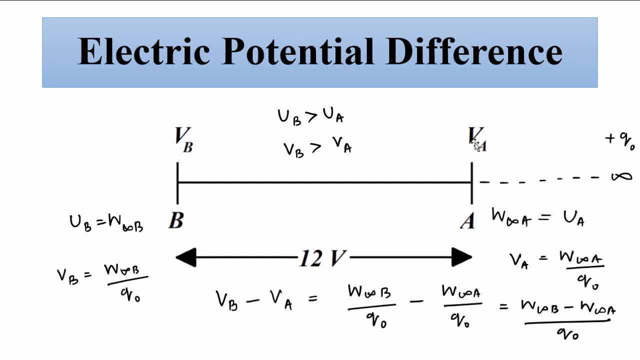 to higher potential point. See VB is at higher potential than A, So the potential difference between these two points is the work done in moving the test charge from a lower potential point to higher potential point against the electrostatic force of repulsion divided by. 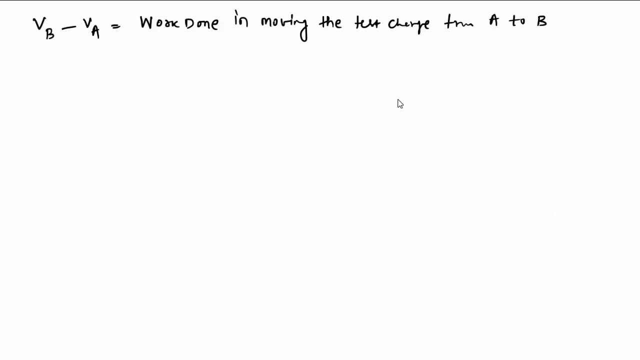 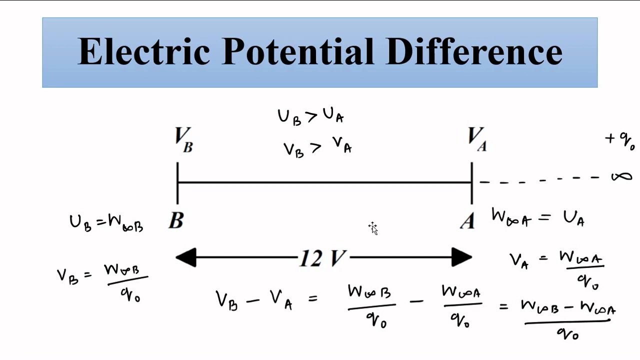 the test charge. So we can also write it as low to high potential point against electrostatic force divided by the test charge value, this test charge value. So always understand whenever we define potential difference. it simply means we have two points which are a different electric potential values. One is at a higher potential, the other one 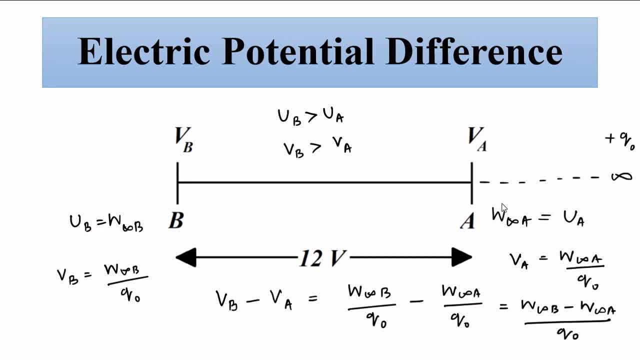 is at a lower potential, the two points- and it simply means the work done against the electrostatic force in moving the test charge from the lower potential point to the higher potential point, Everything which is defined with respect to infinity. So for that first we have to 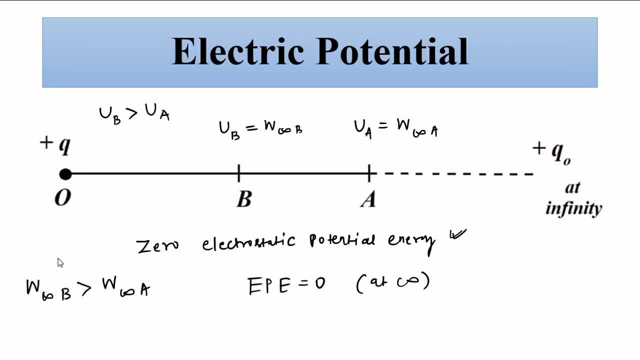 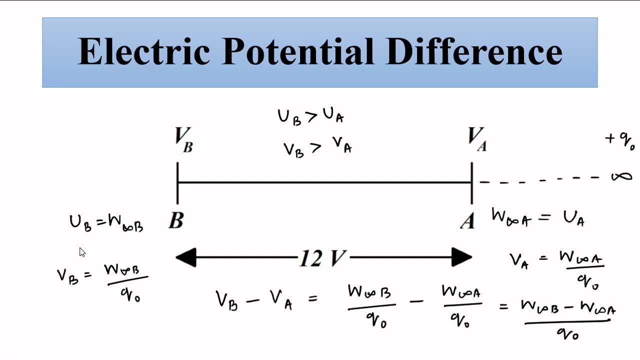 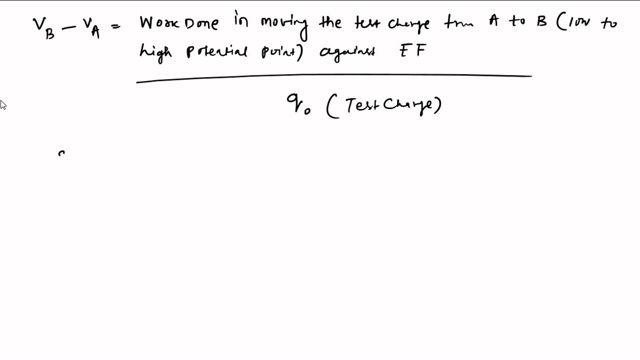 understand electric potential concept, then we can go to electric potential difference. this: So the S? I unit of potential difference is also volt. electric potential: the same thing, one volt. So we can define: S? I unit of potential difference is also volt. So we can say that the potential difference between two points is said to be 1 volt. 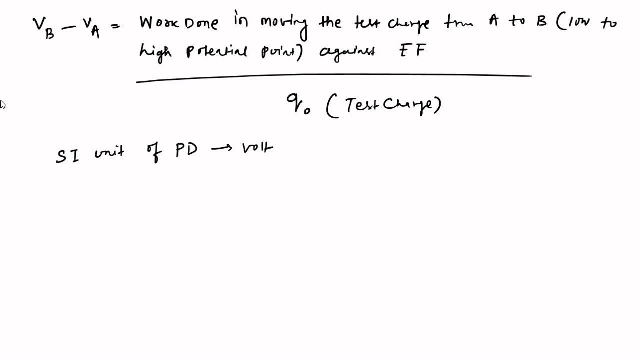 If 1 joule of work is done in moving a charge of 1 coulomb from a lower potential point to a higher potential point against the electrostatic force in the electric field, okay. So 1 joule of work in moving a charge of 1 coulomb from a lower potential point to higher.